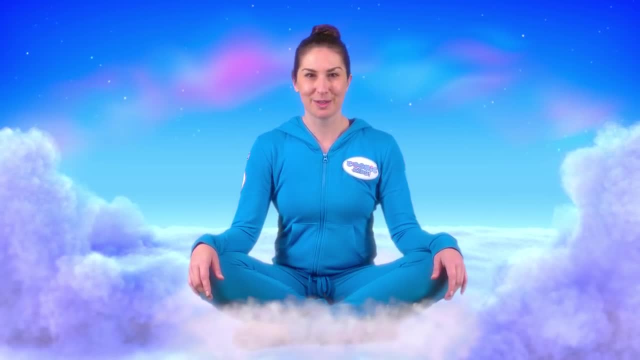 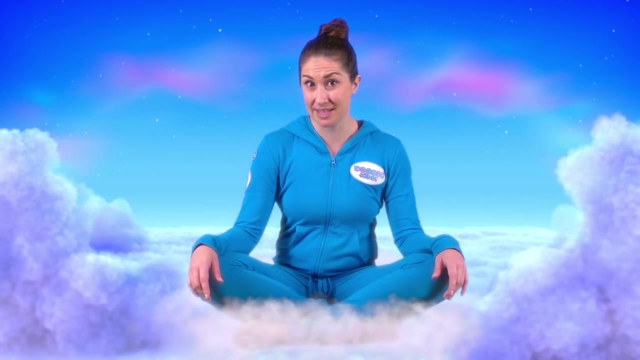 As you come to the Zen Den, more and more you are mastering the most important thing to learn: understanding yourself and how to be happy and enjoy your life. Now I wonder if you can think of a time when you've had to perform in. 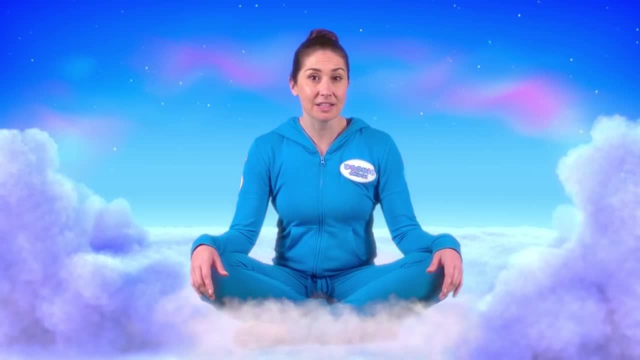 some way. Maybe you've had to speak, act or sing or dance in front of other people, or you've had to play a big sports game at school, or you've had to take an important test. You know it's coming up, the days are ticking by and soon you have to do it. 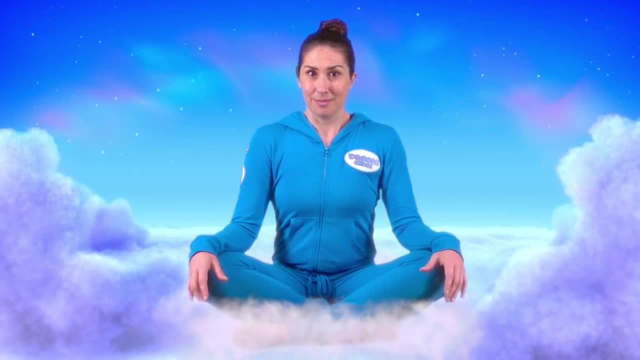 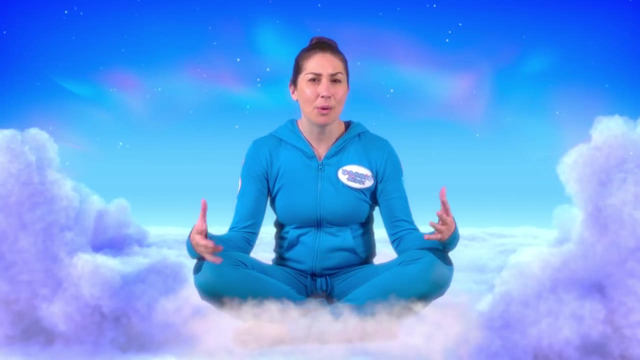 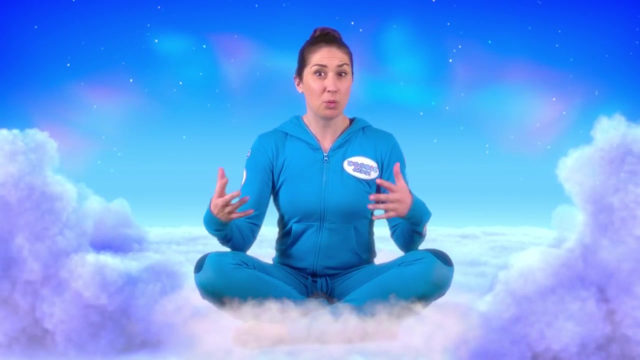 This can feel exciting, but also a little bit frightening. This is what it means to feel nervous. Perhaps you are worried about being looked at or whether what you do will be good enough. Perhaps you worry about what everyone watching will think about you when you do it. 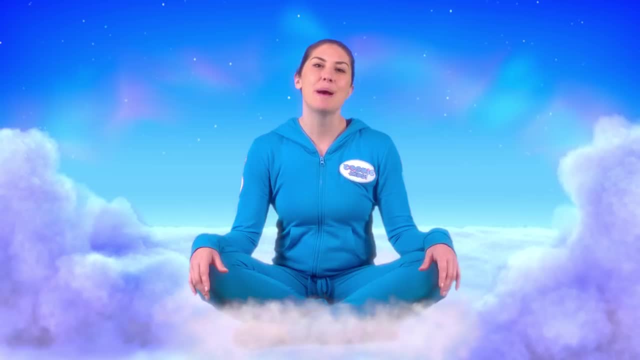 Close your eyes, if you like, and try to remember a time like this when you've had to do something. It might have been a time when you had to stand up in front of your friends in class, or maybe in front of all the kids and teachers in school. 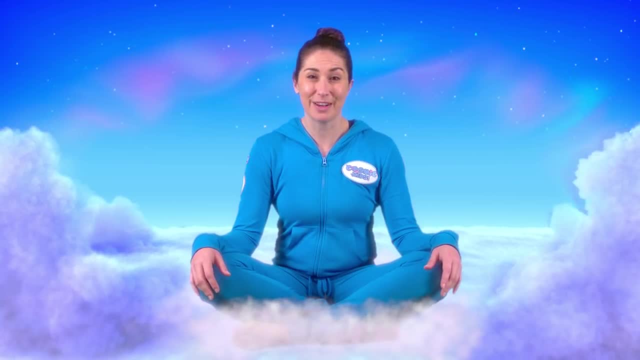 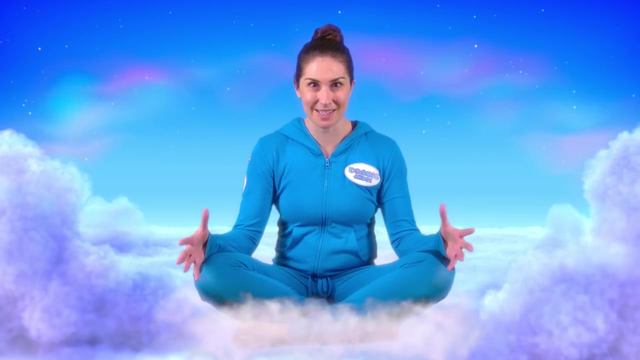 Can you think of one. It's funny even when you think about it now. even though it's past, it's still normal to feel a little nervous. Nervous feelings are natural when we have to perform. We are doing something that is challenging. 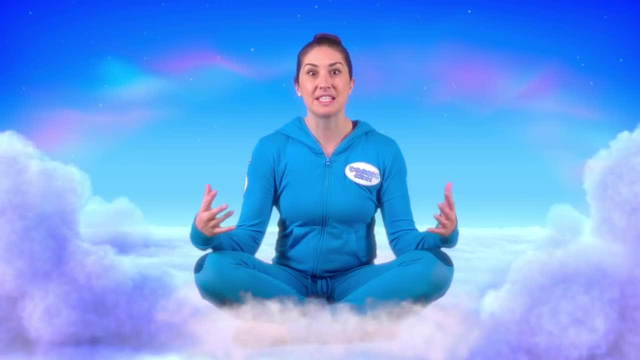 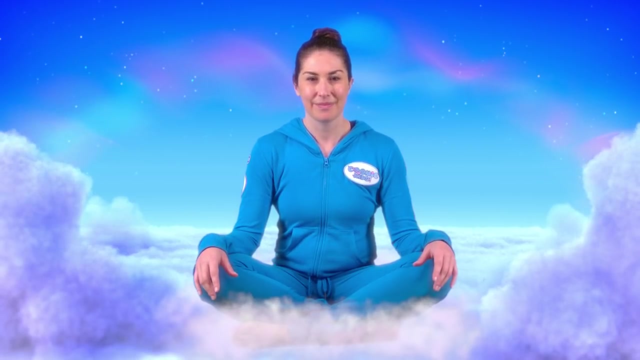 and important for us, something that will help us learn and become better, stronger and smarter We want to do brilliantly. of course, It feels really important and this means we can start to feel nervous. Generally, we feel nervousness in our bodies. Sometimes our heart beats faster. 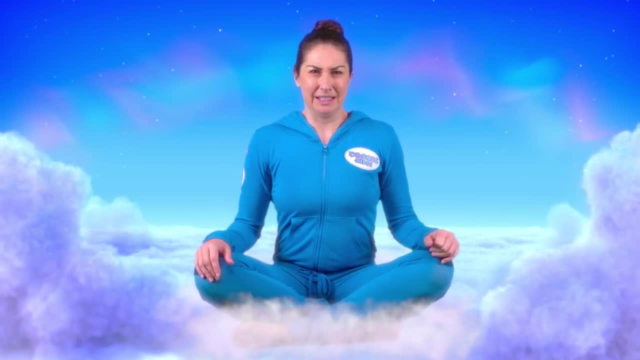 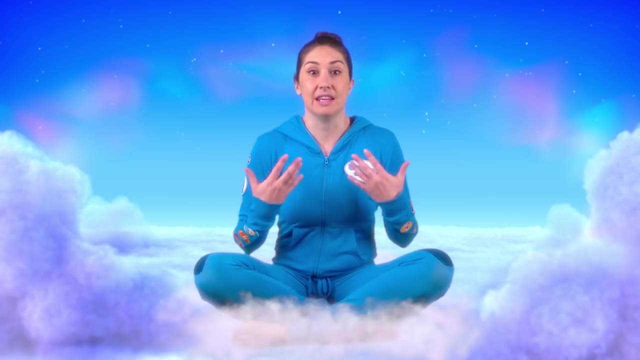 or we might feel like we've got butterflies in our tummy, a kind of wriggling. Another thing that happens is our breathing can become really tight. It's a scary feeling, as if the body is imagining that we're in danger. 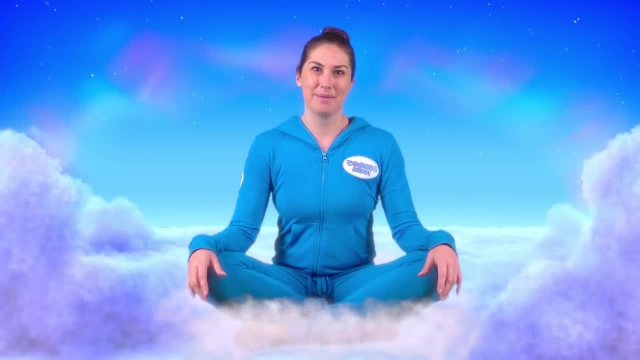 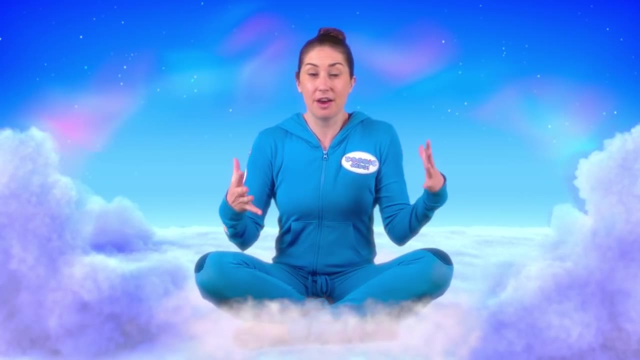 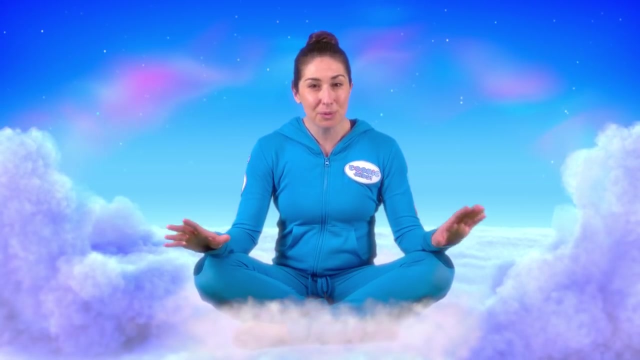 We're not, of course. It just feels that way. The good news is, there are clever ways to balance this fizzy, breathless, nervous feeling with the calmness and focus we need to do our best. If we can be calm, we can keep our heads nice and clear as we do our performance. 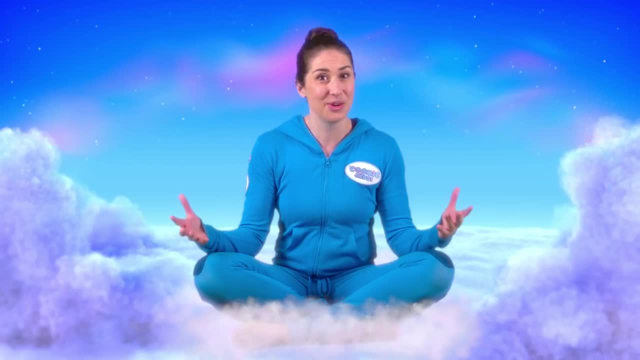 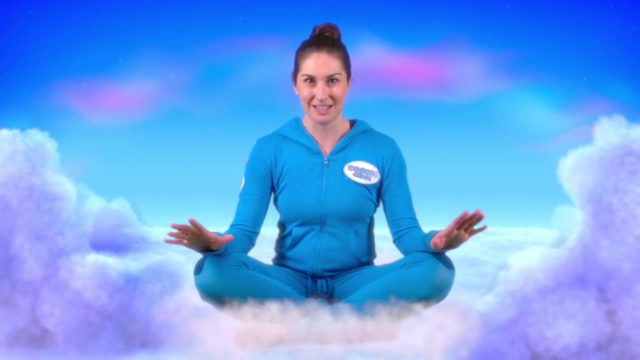 and do it really well and even enjoy it. And this is where your Zen-Den mindfulness practice comes in. We use it to calm ourselves down so we can do our talk or performance brilliantly. Let's try something now that you can use whenever you have something coming up. 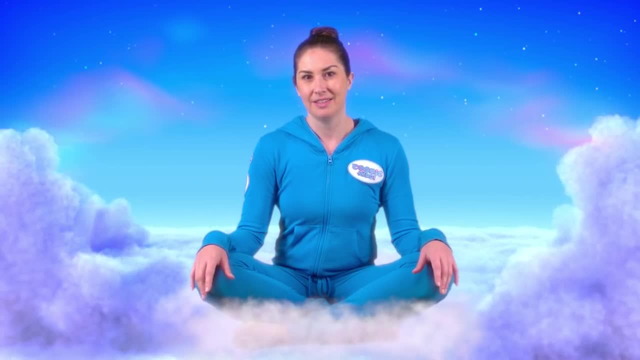 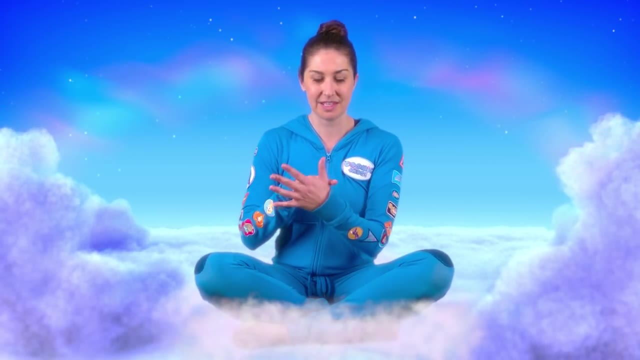 that you need to settle your nerves. I'm going to call it finger breathing. Hold up your hand and bring your finger to the base of your thumb, where your hand meets your wrist. You can use either hand, Close your eyes and breathe out all of your air. 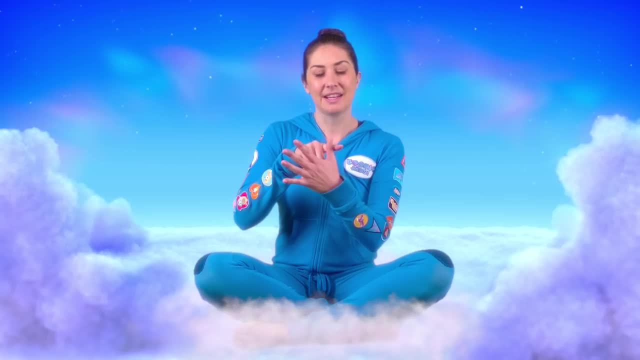 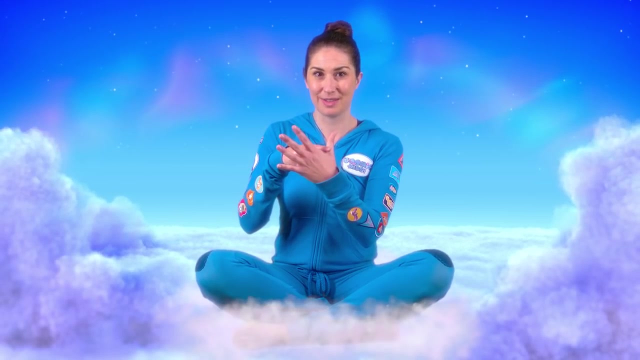 Now slowly start to breathe in and slide your finger all the way up one side of your thumb. When you get to the top of your thumb and you're full of breath, now slide down the inside of your thumb as you breathe out. Let's keep going along our hand. 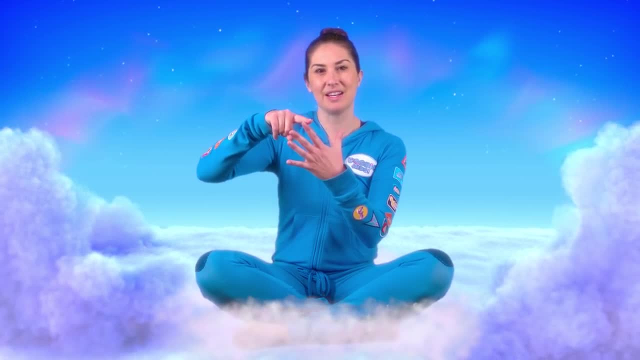 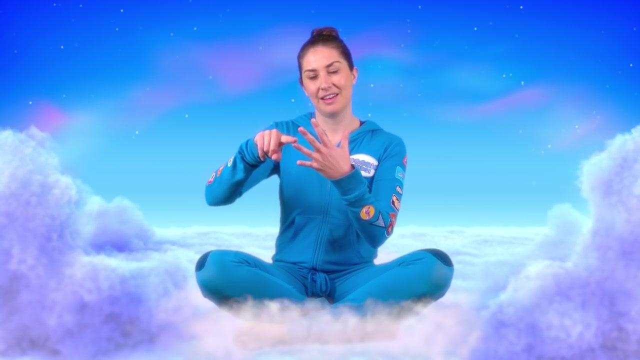 Breathing in as we go up the side of our fingers and breathing out as we slide down the other side. Breathing in, Breathing out, Breathing in, Breathing out, Breathing in And breathing out When you get to the end and your finger reaches the base of your hand. 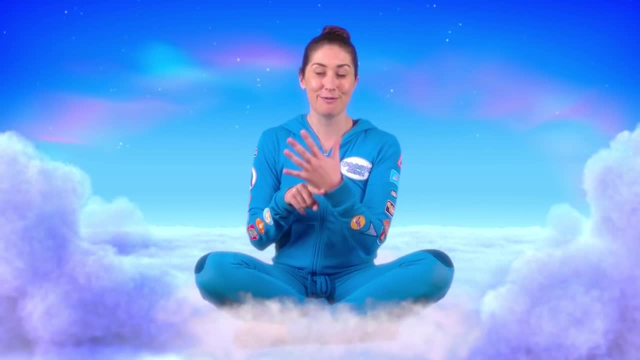 on the little finger side. you'll have taken five lovely, calming, steady breaths. It also feels quite nice, A little bit tickly on the outside and a little tickly on your fingers as you do it, which is good to focus on.